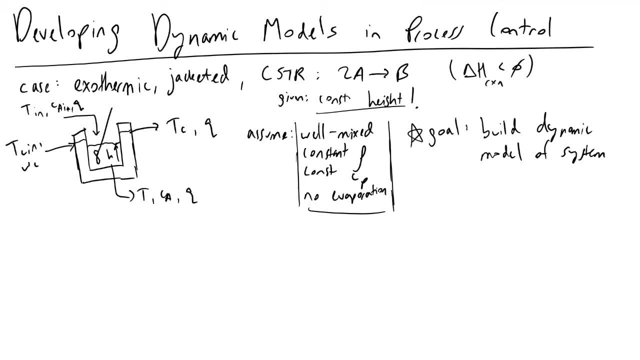 how do you actually go about designing controllers to operate your reactors and keep things from blowing up. So it is pretty exciting stuff And in this video I'll go through how we can go about doing that. And so in this case we're going to be looking at as an exothermic jacketed CSTR in which we have two moles of a reacting to form two moles of B, And because this is an exothermic reaction, heat is being released during the course of this reaction, meaning that delta H of 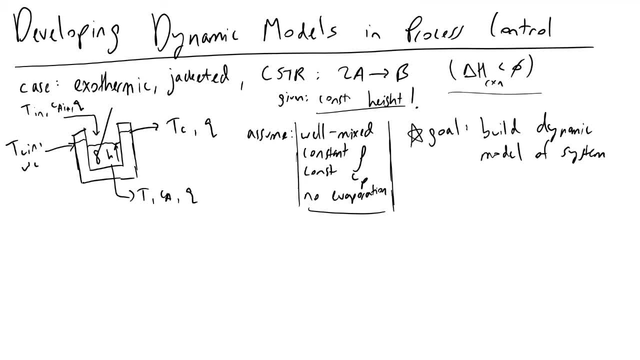 reaction will be a negative value And I drew a diagram of what's going on here So we can keep mind of what's going on here. Tn is the temperature of the inlet feed. CaN is the concentration of A in the inlet feed. we're assuming there's no B in our inlet. Q will be a volumetric flow rate, Ca will have units of moles per volume And we also have a coolant jacket with Tcn going in and Tc 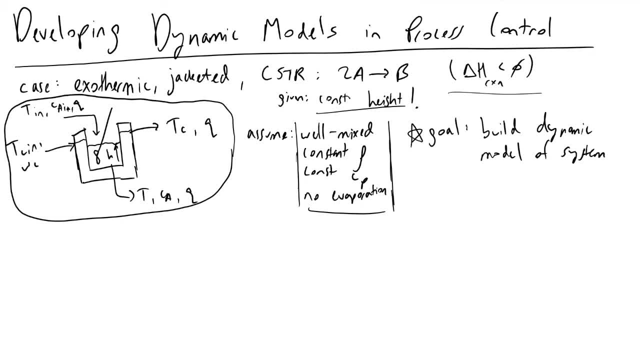 leaving, as well as a mass flow rate of our coolant denoted Wc. And the height of our CSTR is assumed to be a constant during this process, And so we will be making the well mixed assumption, a constant density assumption, a constant heat capacity, meaning that our heat capacity is not some function of temperature, And we will also assume that there's no evaporation occurring. because there's evaporation, the height will change, and 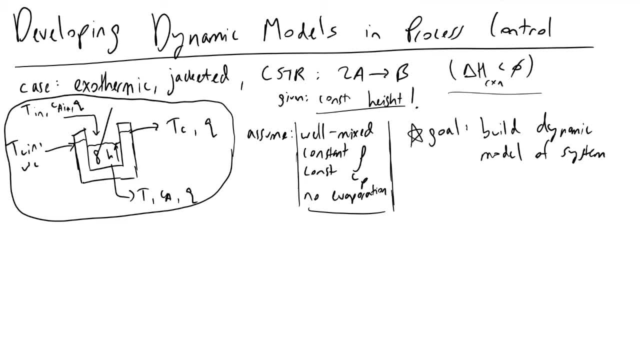 the mass will get a lot more complicated. So, making these assumptions and given this model, our goal is to build a dynamic model of this system, And so, before we do anything, the first thing to ask yourself is: what's changing in our process and what makes process control different from what we've done previously in chemical engineering courses? is that we're not. we're operating at the steady. 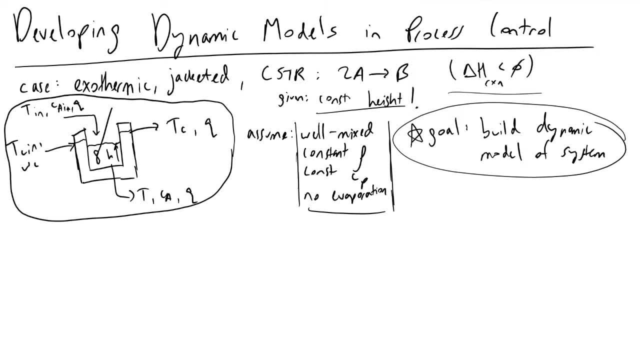 state. most of the time in a process control class. We're interested in startup behavior, shut down down behavior, And so a key note here is: we're not at steady state usually, And so canceling out the accumulation term that many of us have become very used to is no longer going to apply, And so 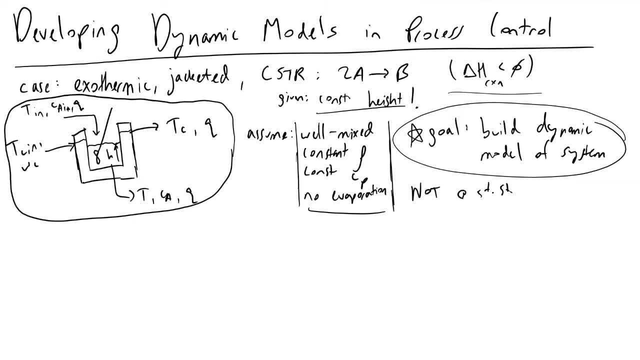 in all of our dynamic models, we will keep the time derivative component of our terms And so, moving forward, what we see is the big question is: what's changing in our system With respect to time And another way of phrasing that is, what do we care about? And 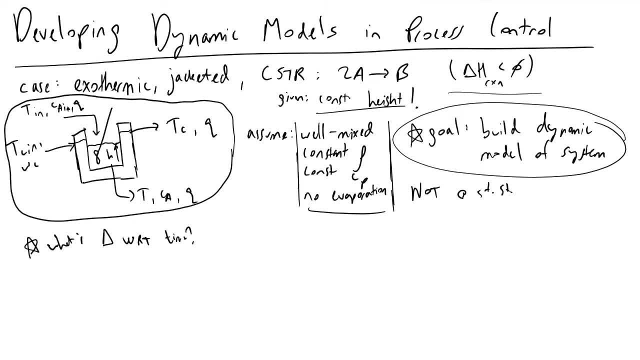 so, intuitively, we care about four things in this process. One: we care about the concentration of A, we care about the concentration of B, we care about the temperature of our reactor and we also care about the temperature of our coolant. 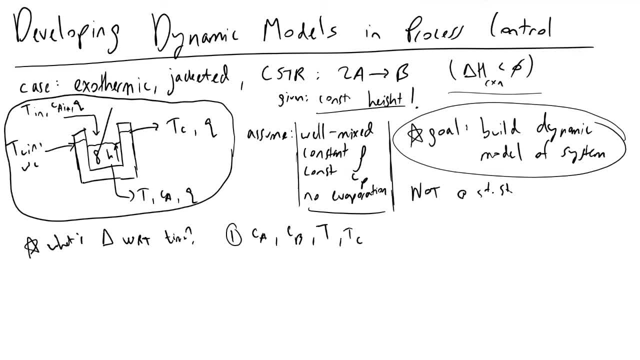 And these are four parameters or values that will be changing as we feed in A, as our reactor is starting up or shutting down, or even operating as it normally is, because there are perturbations that are occurring, And so what we're going to do is start turning to our mass balances and our 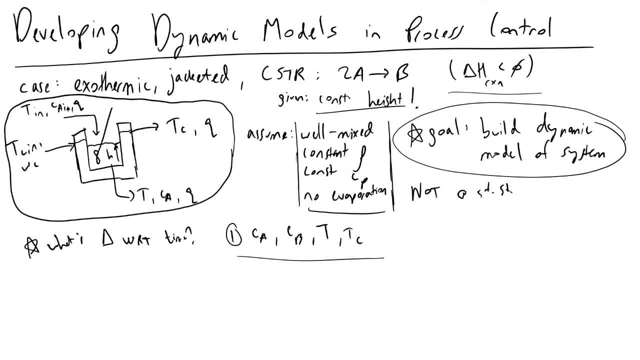 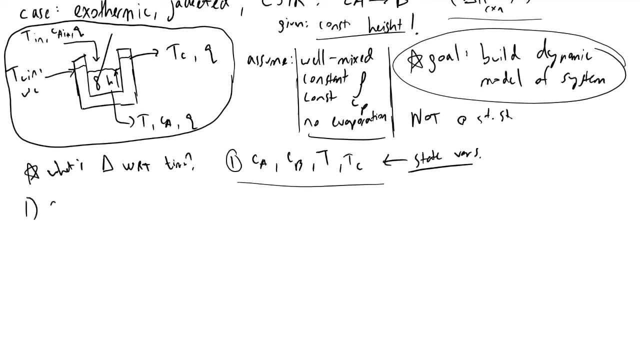 energy balances to derive four equations that are associated with each one of these state variables. State variables is another term that we use frequently in process control to denote anything that's changing with respect to time and we care about. And so the first one, CA. we're going to turn to a mole balance, an overall mole balance of CA in our tank. 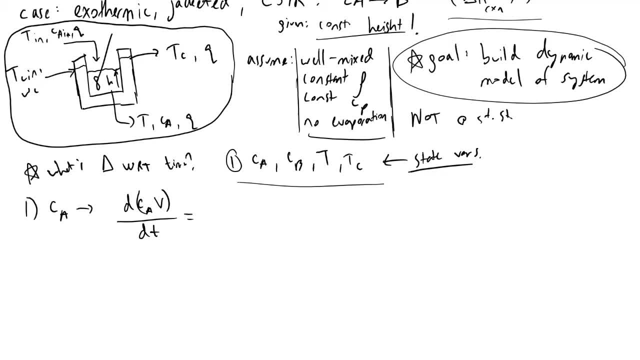 So the change in A with respect to time- and this is equal to DNA DT number of moles will be equivalent to the number of moles that are entering our reactor as a function of time. so we'll have CA n times Q leaving our tank, we will have CA times Q and we also have CA reacting and 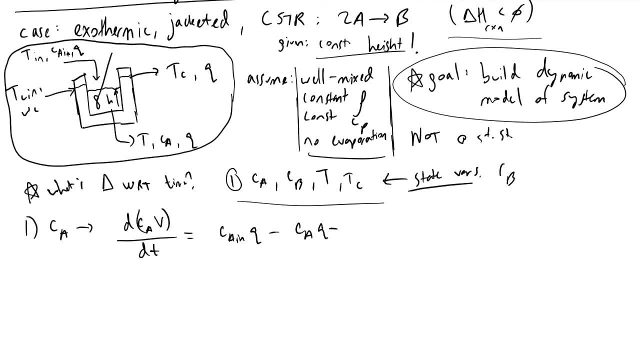 another thing I forgot to note here is that we are given the kinetics of our system, which were determined to be K naught times, some exponential, and then the activation energy of A divided by the temperature times, CA squared, and this has units of moles of B per volume, and so we need to recognize that. 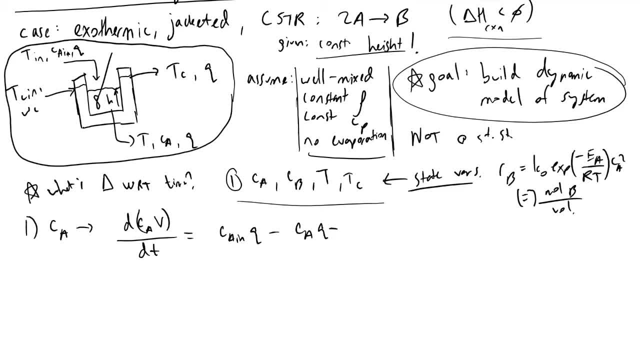 this is the number of moles of B that are consumed. for every mole of B that was consumed or produced, we had to consume two moles of A, and so we will have two times RB, times our reactor volume, V. and it is another common thing, just to keep the 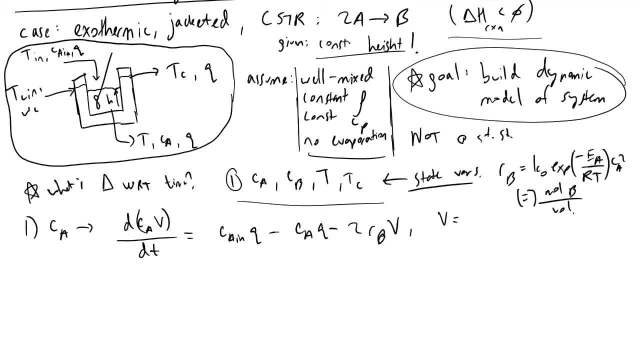 math a little bit cleaner is: we'll let V be equal to some cross-sectional area AC times a height H. the nice thing here is that we were given at our height is constant, so we have to worry about that and we have to be careful. we're using a constant constant to do that right now. 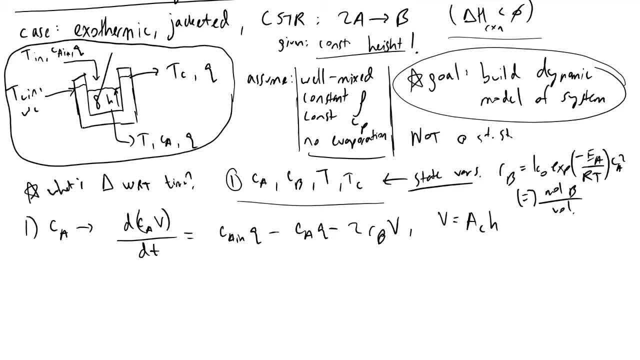 and so we're going to, we're going to have to do that, we're going to have to have to do that and we have to be careful. so we're going to have to think about these numbers and so, now that we know that, we have the next step if we move. 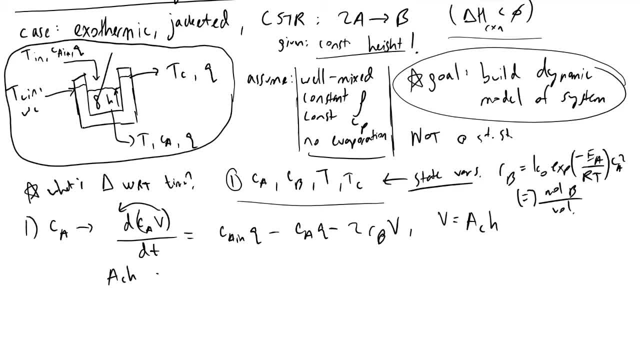 on to the next step and further evaluate this. we can pull out V here, so we'll recognize that DC a, V, dt, because V as a constant comes out of our derivative, and so now we have a C times H times DC. a DT is equal to CA n times Q minus CA times. 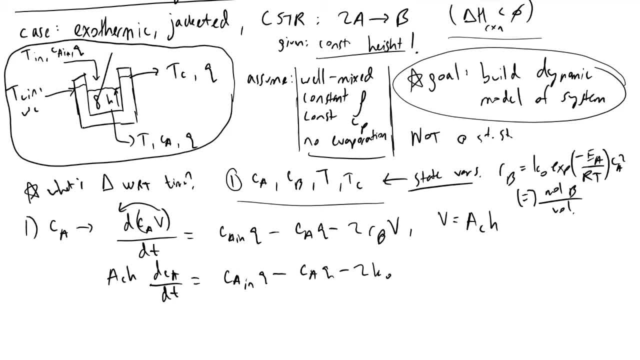 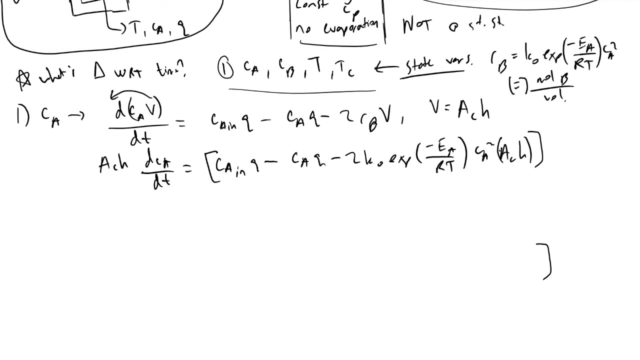 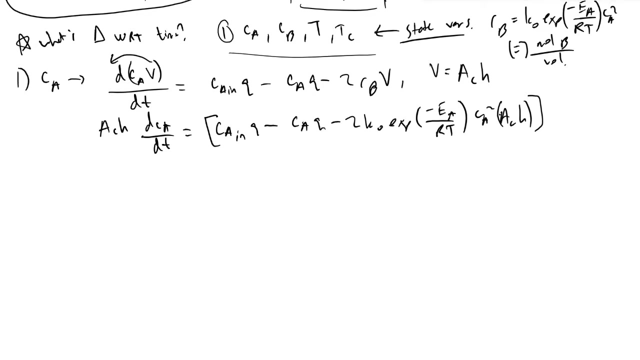 times K, naught exponent minus Ea over RT times Ca, squared times the reactor volume V, which we established to be Ac, times H, And we can isolate at this point dCa, dT, Sorry, one sec. And so if we divide both sides of our equation by Ac, 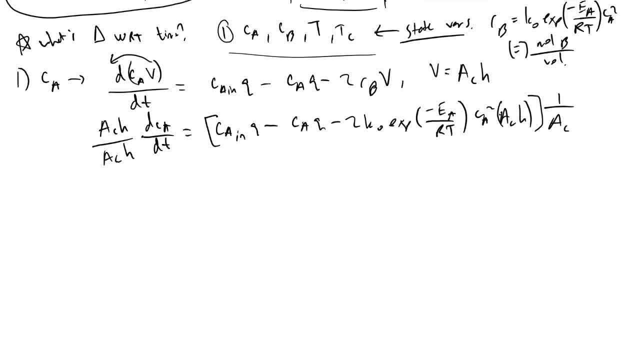 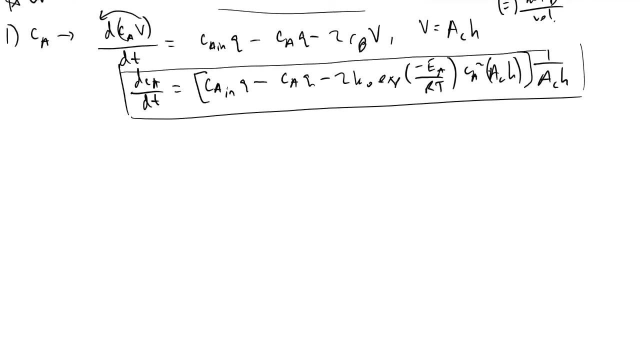 times H, 1 over Ac times H. we can isolate dCa, dT like, so Sorry. And the next thing we're going to look at is mole balance on B, to see how its concentration is evolving with respect to time. So we'll have the same form, dCb. 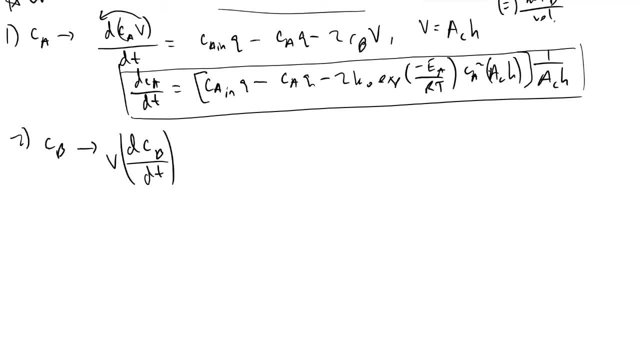 dT. I'm going to pull out the volume just because we did previously And we'll assume we have no moles of B entering our system. We do have moles of B exiting our system And we also have a rate of formation. 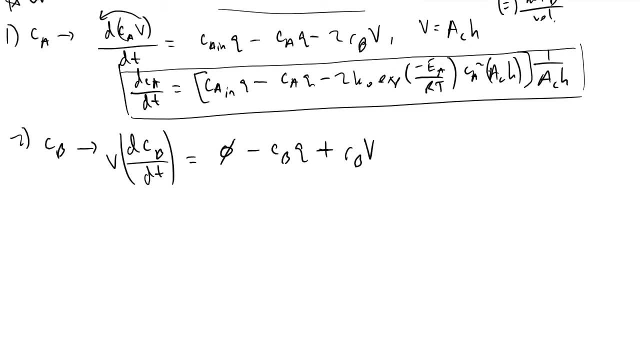 So we're going to have a rate of formation of B exiting our system And we also have a rate of formation of B exiting our system, And we also have a rate of formation of Rb times V And if we plug In these values and simplify, we will end up getting dCb. dT is equal to: 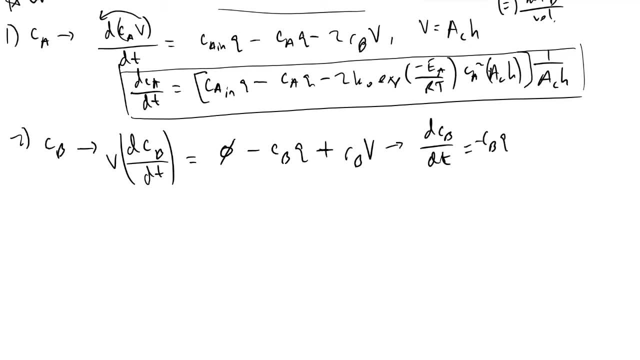 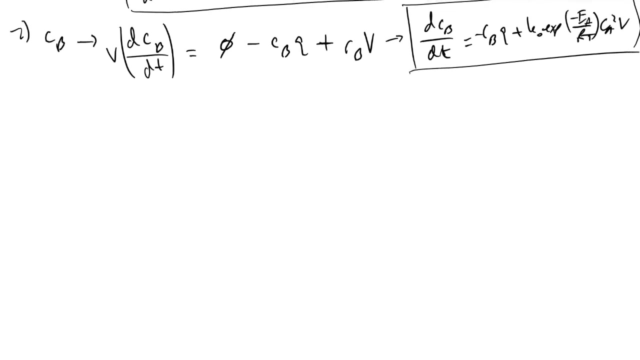 Cb minus Cb times Q plus k. naught exponent minus Ea over RT Ca squared times V. The next thing we are interested in is the temperature of our reactor as a function of time, and this I shall call T, and to do that we're going to turn to an. 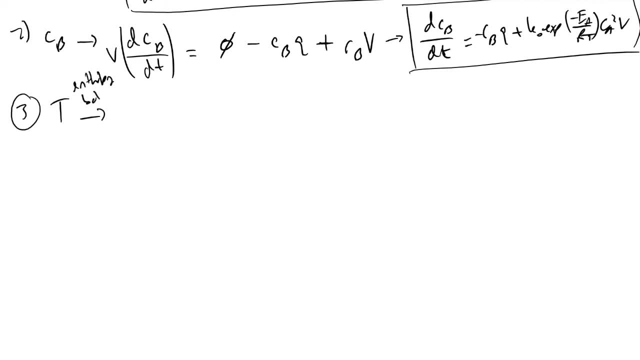 enthalpy balance, as we'll call dH, is equal to mCp dT. so this is what we're going to be working with, and so, if we begin to analyze this, what we'll have is dH. dT is equal to dmCp t- dT, and the mass of our reactor was equal to rho times V. 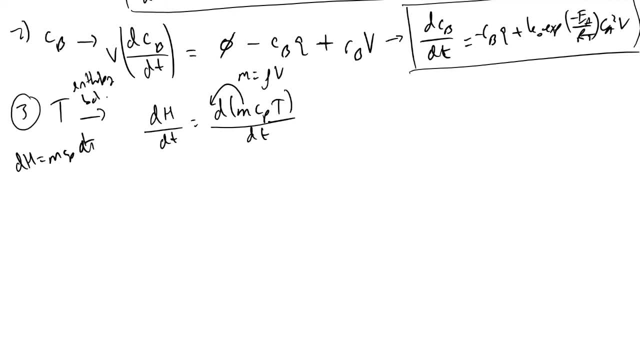 we made a constant density assumption and a constant volume assumption, so we can pull out m, and we're also going to make an assumption that Cp is temperature independent, which also makes it time independent. so we can pull out Cp as well and we get rho V, Cp, dT, dT is. 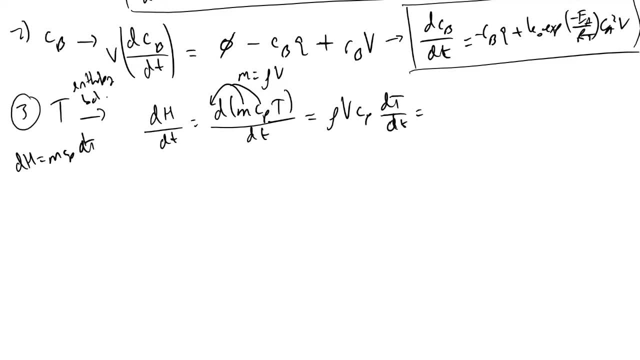 the accumulation of enthalpy in our system, and this I'll rewrite down here because it gets a bit long: rho V, Cp, dT, dT, dT is equal to the enthalpy coming into our system which will have the form: rho times Q, density times, the volumetric flow rate is equivalent to the mass flow rate. 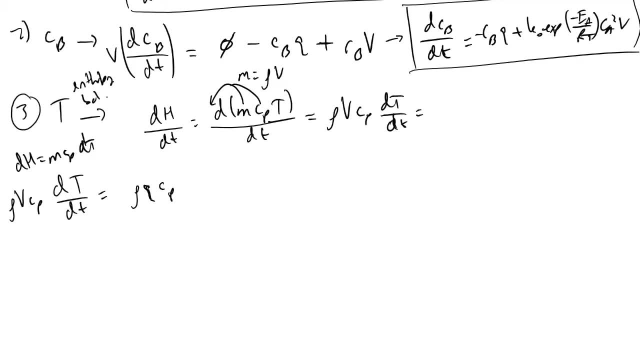 times the Cp, the heat capacity of our system, times T in, that's enthalpy coming into our system and then we'll have enthalpy leaving our system. so rho Q, the mass, and then times Cp, times TL, and then we're losing energy to our heat jacket. minus UAH, so an overall heat. 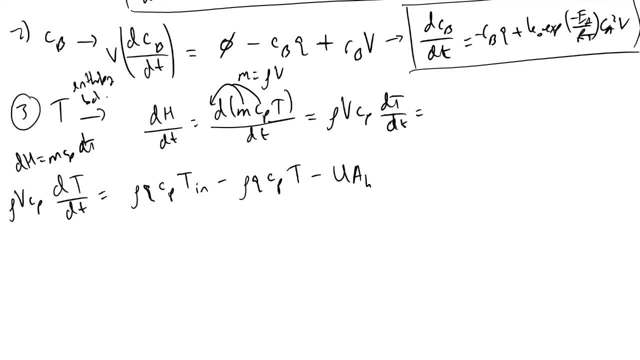 transfer coefficient times AH, which I call the interfacial area between the jacket and the reactor, and then the temperature difference, which is the driving force for heat transfer- T minus TC, the temperature of the coolant, and we also have a heat of reaction term occurring, because we're dealing with an 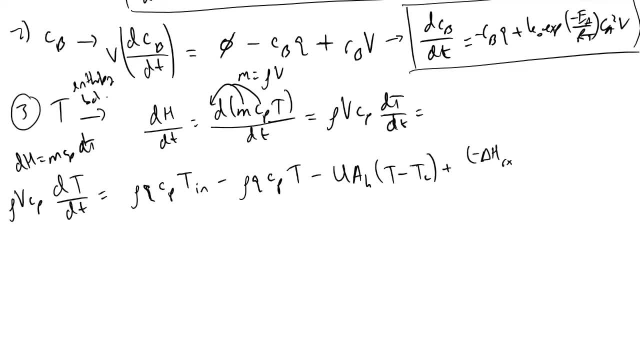 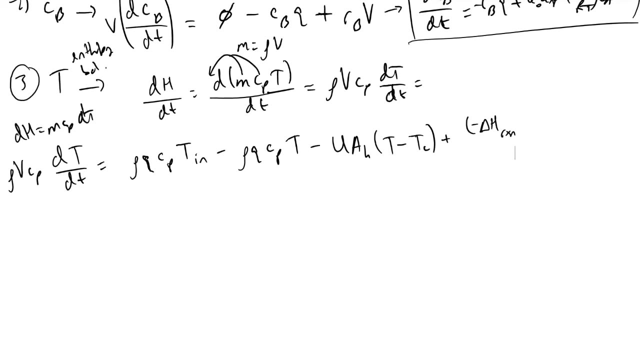 exothermic reaction. so this is equal to minus delta H reaction. because delta H was negative, we need to throw this other negative here, because temperature will increase as more moles of your exothermic reaction react. sorry, and we're going to multiply this by the rate of reaction to get energy per time and 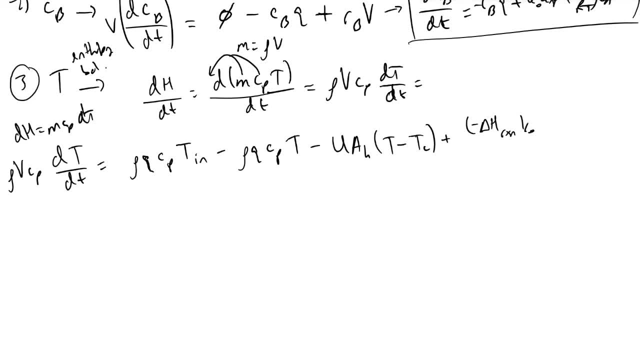 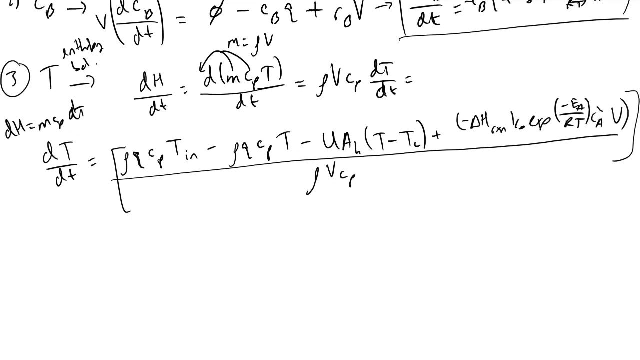 that will have the form of K naught exponent minus EA, over RT times CA, squared times V, and so now, if we divide all of these terms by Rho V, CP, we can arrive at a- sorry, yeah, final form of our how our temperature is evolving with respect T time in our reactor and finally, what we're going to do is turn. 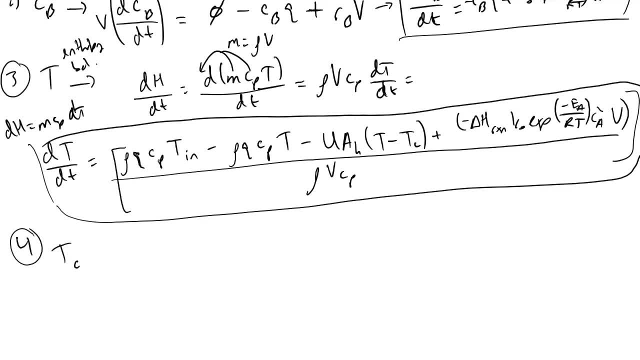 to the temperature of our coolant jacket, and again we're going to use another enthalpy balance, but this time we're going to be doing it on the coolant. so dhcdt is equal to, and in this case we've got the following: where we have dhcdt equal to, 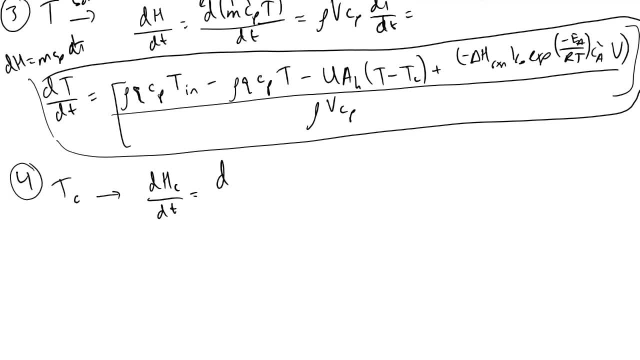 have, DHCDT is equal to D times MC, CPC, TC, DT, and we're going to make the assumption that the coolant height or the mass of coolant in our jacket is constant over time, so we're going to pull that out, as well as the heat capacity, and so this is really equal to MC, CPC, DTC, DT, and if we now perform, 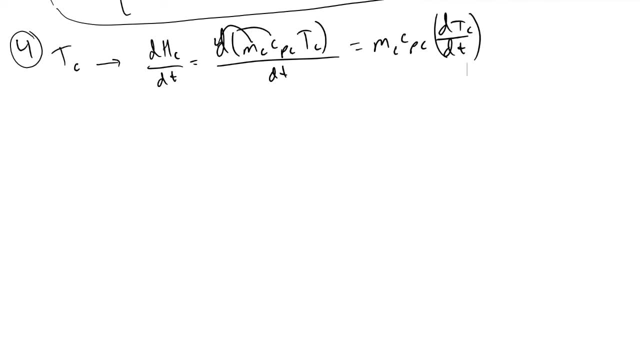 another enthalpy balance on our system. what we will arrive at is we'll have MC, CPC, DTC. DT is equal to WC, the mass flow rate of a coolant times its heat capacity, CPC times the inlet temperature of the coolant. TC in and then leaving. we'll. 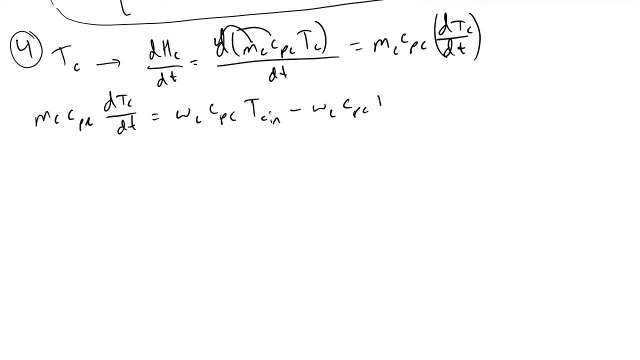 have WC, CPC, TC, and then we also have energy coming into our coolant thanks to the heat jacket or the heat transfer, which is UAH times T minus TC, and if we divide all of this by MC, CPC, we can cancel out these terms. on this side, we end up with our equation that 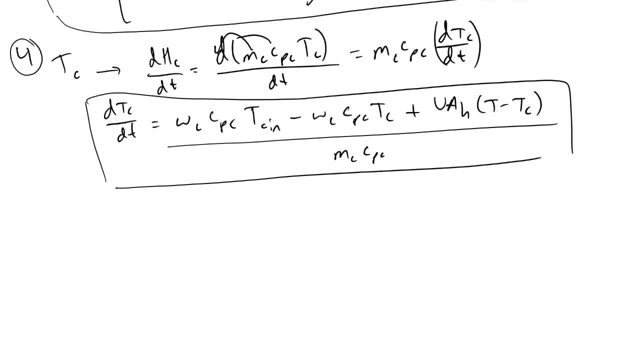 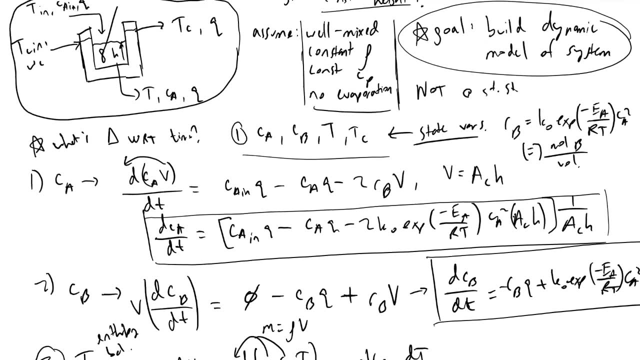 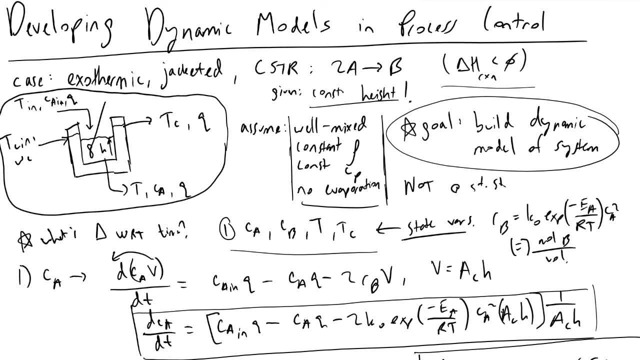 tells us how the temperature of our coolant is evolving with time. and so what we're able to do is arrive at these four equations that tell us how our exothermic CSTR is evolving with time. and this is the first step in a process control class. the next thing we're going to do is princess control class. the next thing we're going to do is accicion control and then attractive feedback, and I'll move the result: Soyacetaseöl attack against it is equivalent, whereas here we do have the same process. 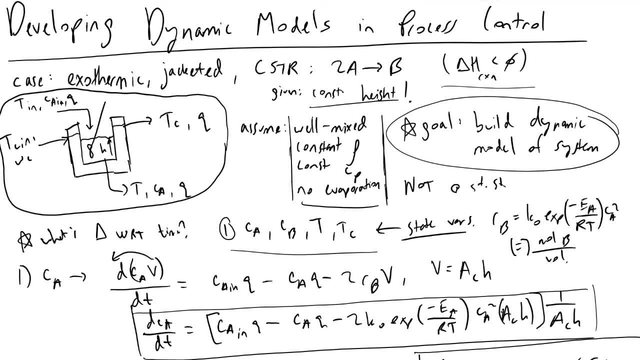 the next thing we're going to do is put these into state space and do Laplace transforms that will allow us to build process transfer functions out of them, so that we can actually begin to make feedback controllers to control these kinds of processes. and so this concludes how we're able to do that: make the dynamic models. I hope you guys find it useful. let me know if you have any.